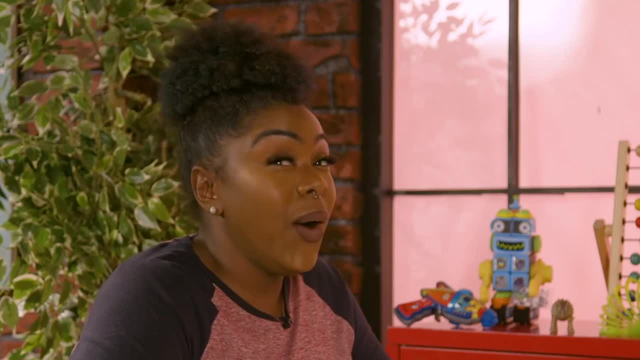 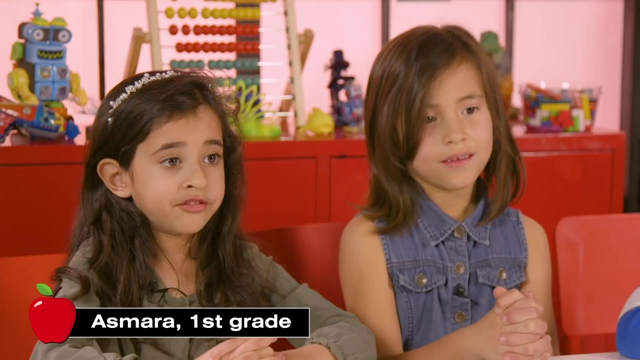 Hey, how's it going? I'm Destiny And I'm gonna crush you. Oh okay. Hi, my name's Asmara and I'm in first grade. Hi, my name is Lyndon and I'm in third grade. 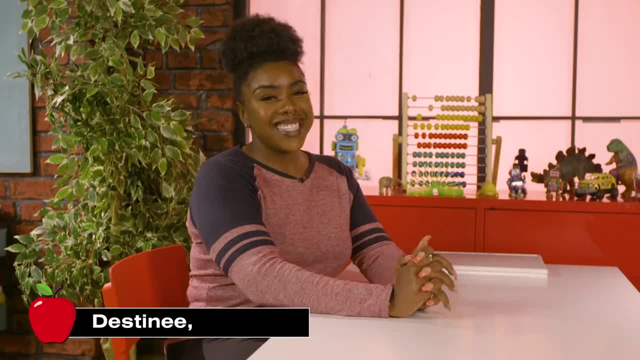 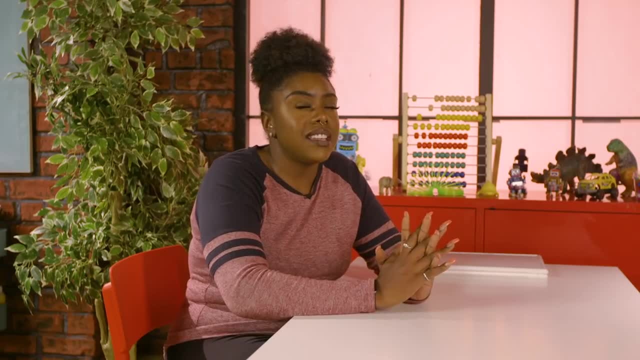 Hi, my name is TJ and I'm in fourth grade. Hey, I'm Destiny and I haven't been in school for I'm not gonna say how many years, but more years than they are old. My relationship with math is a love-hate relationship. 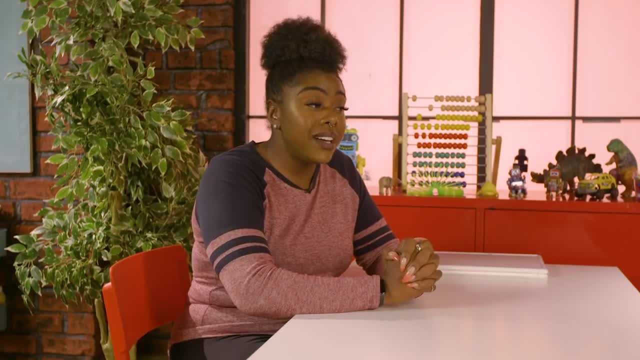 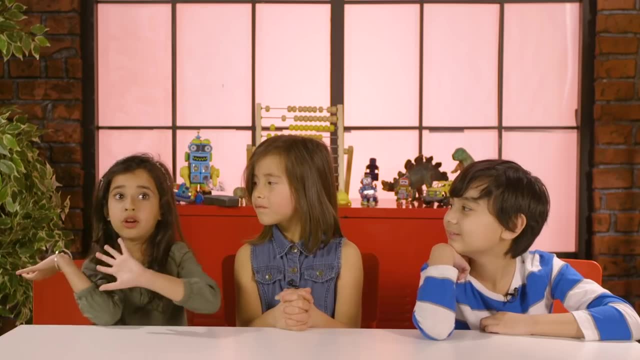 I actively avoided taking math classes And that's how I ended up in journalism. I'm good at math. I'm really good. I'm good at math. I think I'm gonna beat my competitor. They don't remember that much of their childhood. 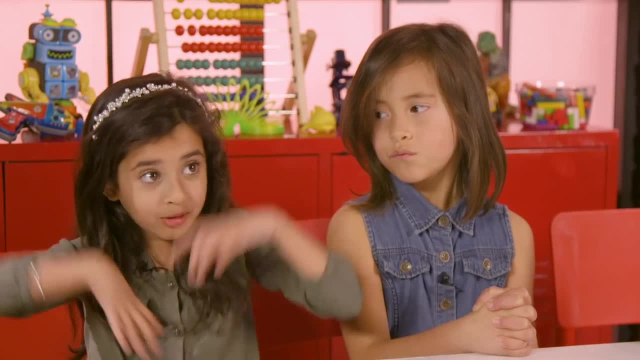 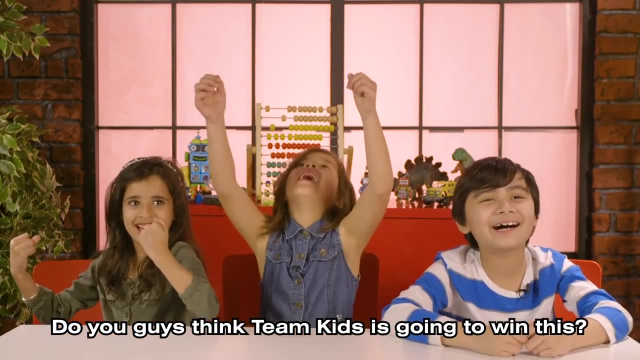 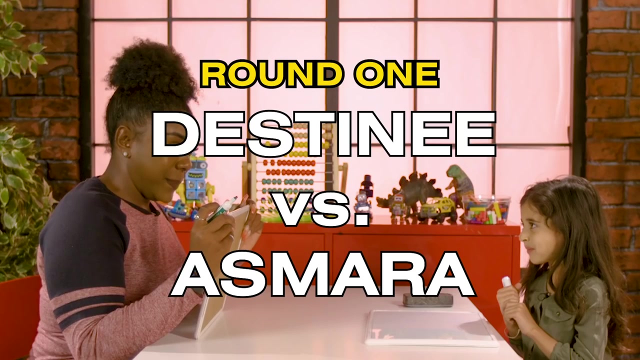 but they know a lot of their grown-up so they'll forget all the math. Yeah, Exactly. No, that's no Exactly. Do you guys think Teen Kids is gonna win this? Yeah, No, No, No, No. 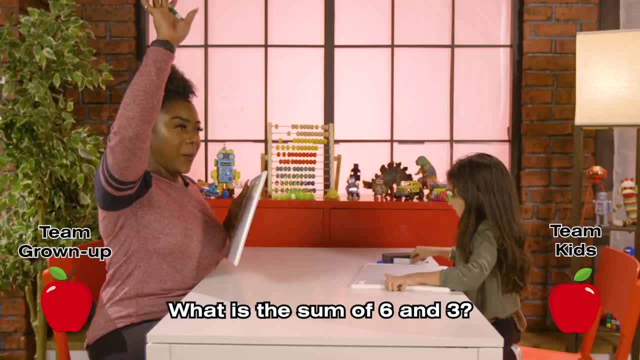 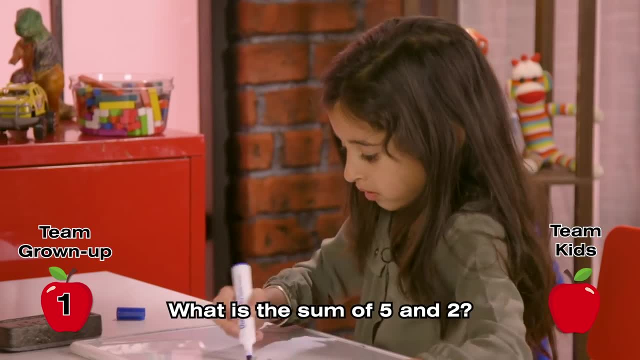 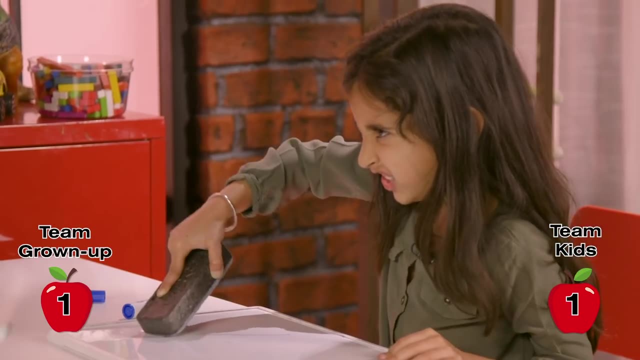 What is the sun sum of six and three, Destin, Is it nine? Hooray? What is the sum of five and two? I'm still writing five plus. That's fine, That's fine. One for one, Wow. 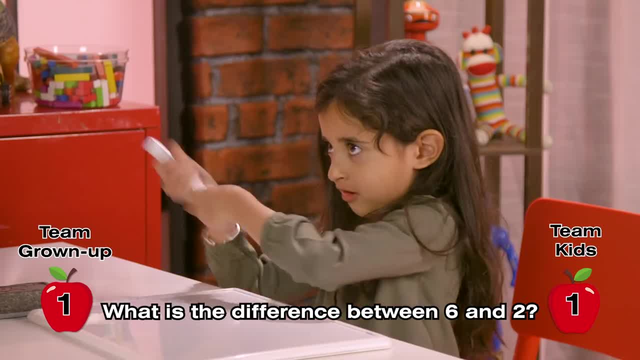 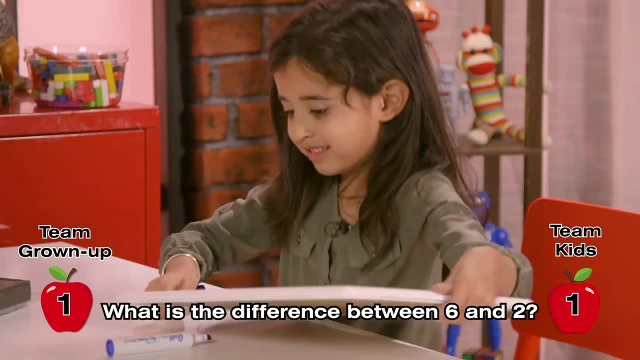 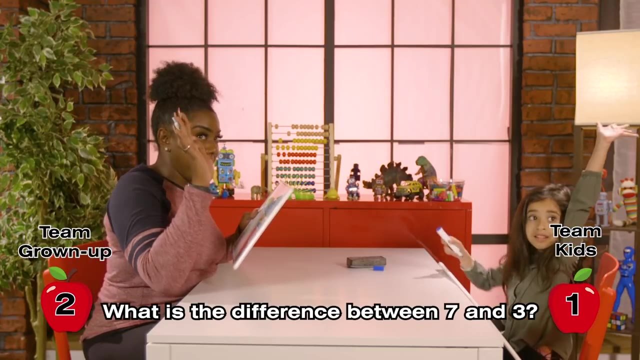 Thank you, Oh, I'll just wipe it with my finger. Oh, that's Babe. Six and two. Wow, One, two, three, four, five, six, seven, eight, nine, 10,, 11,, 12,, 13,, 14,, 15,, 16,, 17,, 18,, 19,. 20,, 21,, 22,, 23,, 24,, 25,, 26,, 27,, 28,, 29,, 30,, 31,, 32,, 33,, 34,, 35,, 36,, 37,, 38,, 39,, 40,, 41,. 42,, 42,, 43,, 44,, 45,, 46,, 47,, 48,, 49,, 50,, 51,, 52,, 53,, 54,, 55,, 56,, 57,, 58,, 59,, 60,, 61,, 62,. 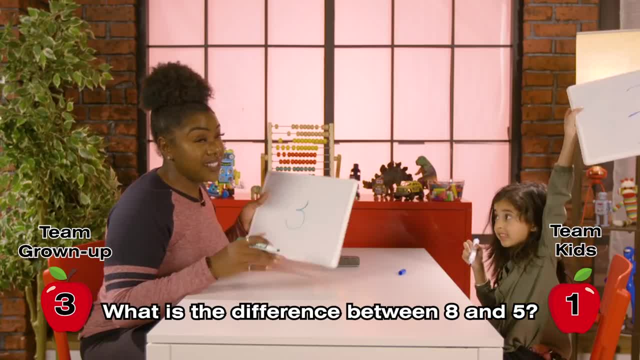 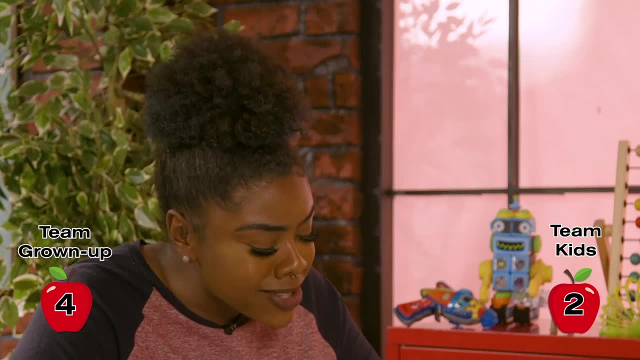 62, MORE: 52,, 53,, 54,, 55,, 56,, 62,, 62,, 63,, 62,, 62,, 63,, 62,, 63,, 64,, 65,, 66,, 67,, 78,. 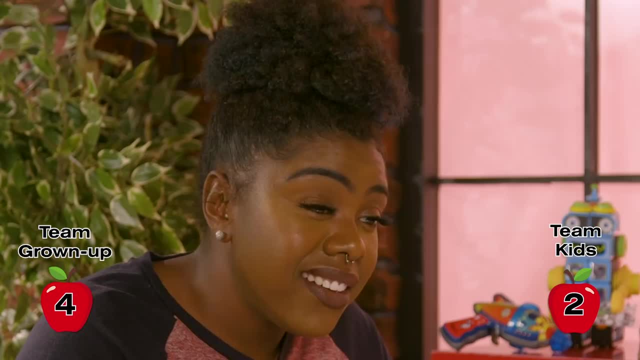 78,, 69,, 79,, 80,, EIGHT, 91,, 92,, 93,, 94,, 95,, 96,, 97,, 80,, 91,, 92,, 93,, 94,, 93,, 94,, 95,, 96,. 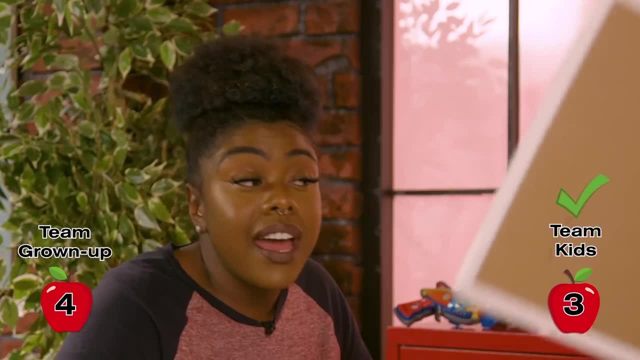 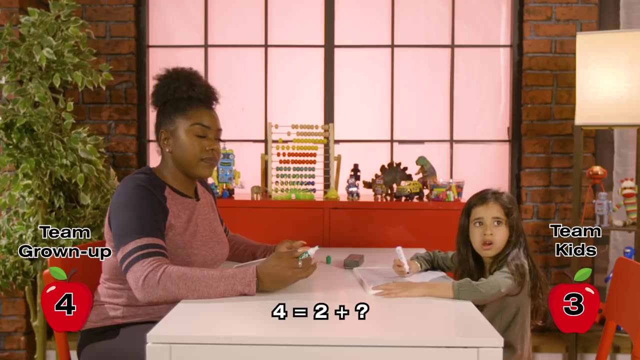 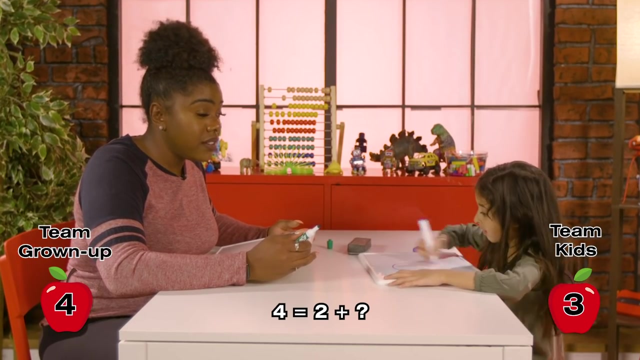 lehc. ¿So we're paying this, not confidently, 05.. Well, she did show hers. It's the points of a square like one, two, three, four. Oh, Four equals two plus what number Do you know that one? 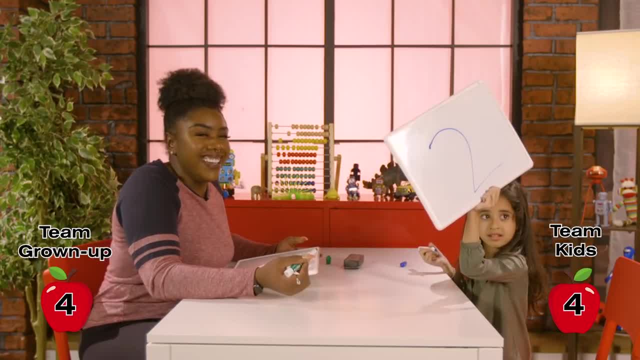 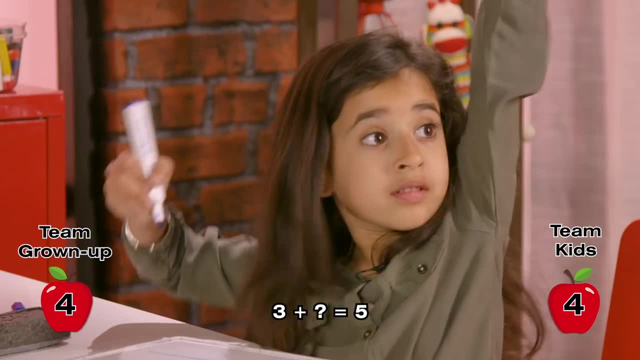 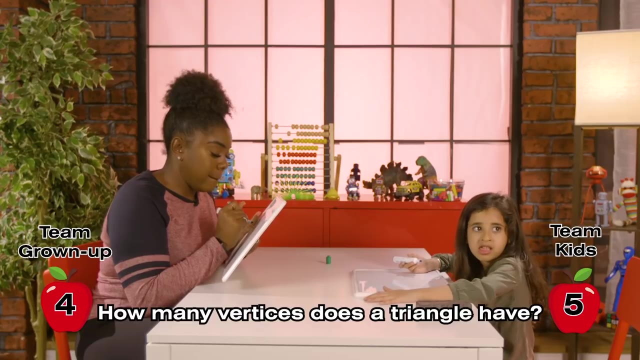 Oh, four. We're doing it backwards. Why Math is hard forwards. Three plus what number equals five. Asmara, I need to write out equations. You are on it. How many vertices does a triangle have? Because she taught me what vertices are. 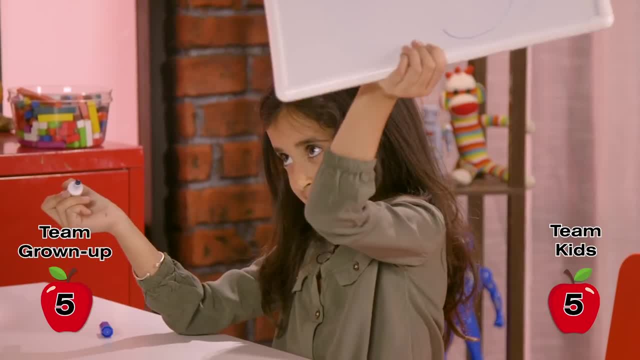 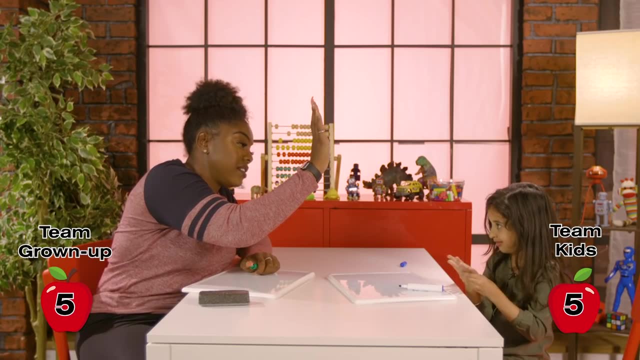 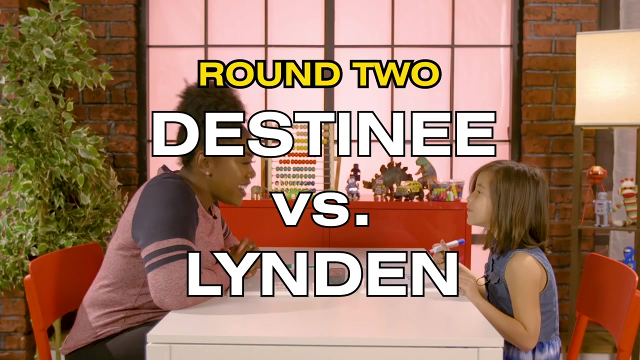 There are three. I only got this because of you. It's a tie. Yeah Well, you did great High five. You also taught me something, So, oh, that one Got it. Hey, how's it going? 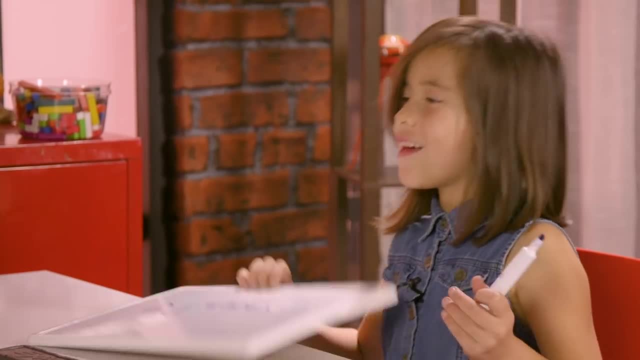 Good, Good, I'm Destiny. It's nice to meet you, Hi. Hi, I am Lyndon Lyndon. OK, Are you ready for our math quiz today? Yeah, I don't know The last person. they took me by surprise. 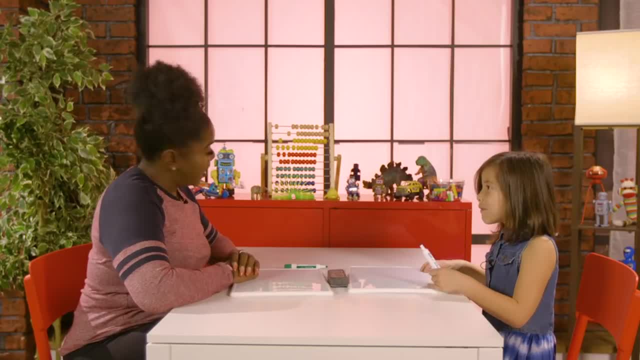 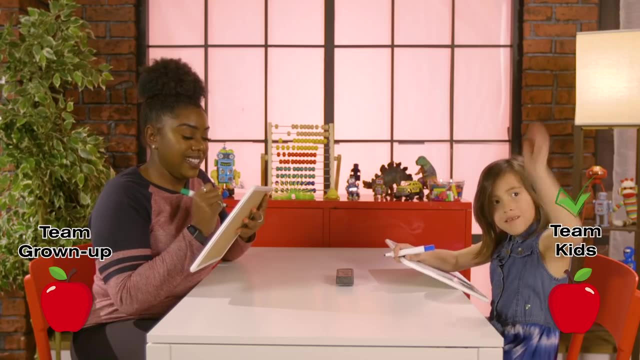 So I'm kind of nervous. Are you going to go easy on me? No, OK. Well, I believe y'all are consistent. What is 4 times 8?? No 32.. Correct, Good, I got 4 times 8.. 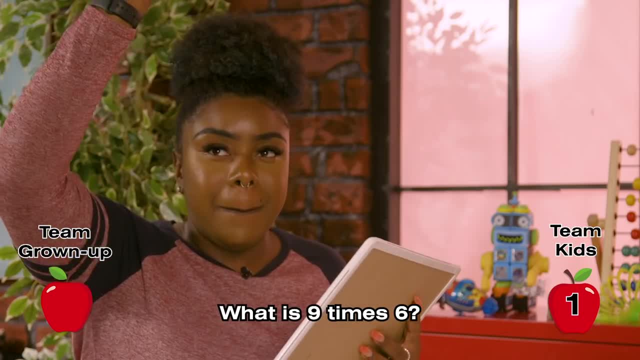 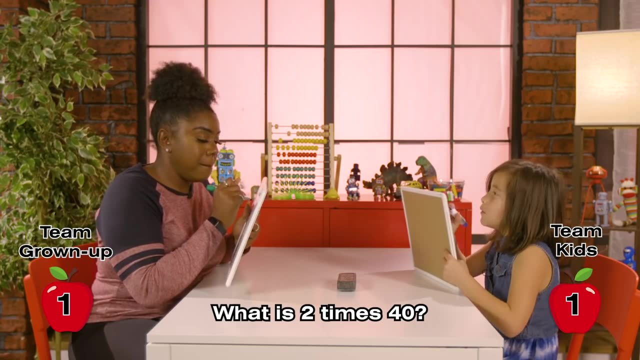 What is 9 times 6? Destiny, Let me finish: 54.. Correct, Woo, Ah, Woo Woo. 2 times 40.. 2 times 40.. 80.. Oh, Oh, Oh Yeah, Raise your hand. 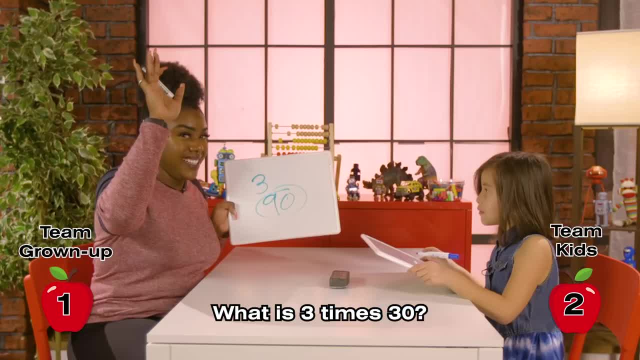 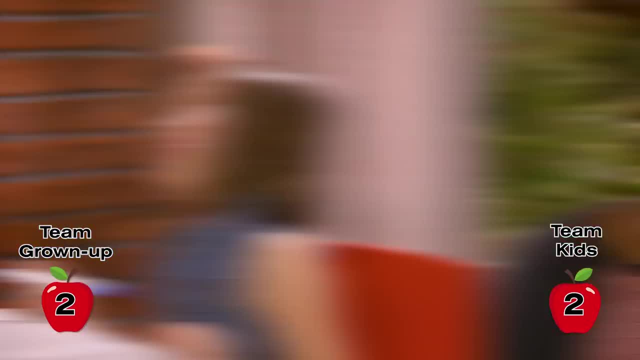 Yes, Yes, Is it 90?? Woo, Oh no, Puffy, poof, poof, poofy, Not even English. 12 divided by 4.. Huh, huh, huh, huh. 3,, 3,, 3.. 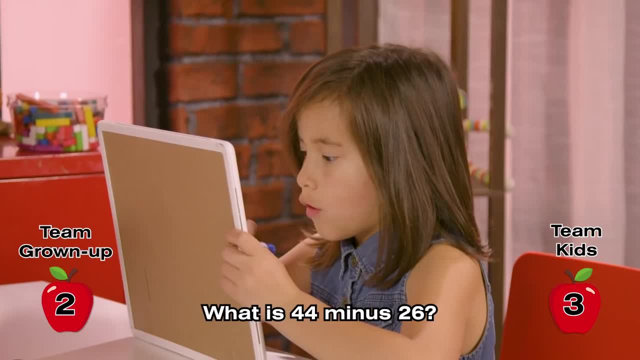 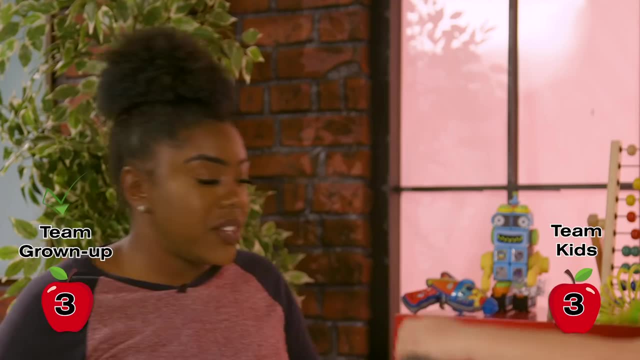 I followed the rules. No, no, no, no, 1.. OK, OK, OK, OK, Is it 18?? Woo, Did you get there? Oh, you have it Y'all. that was a lot. I was like: no, the 3 is not a 1.. 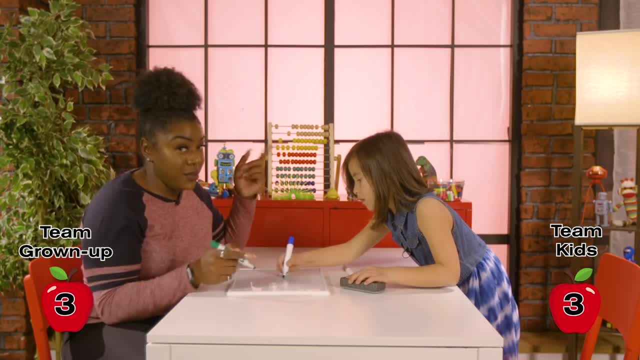 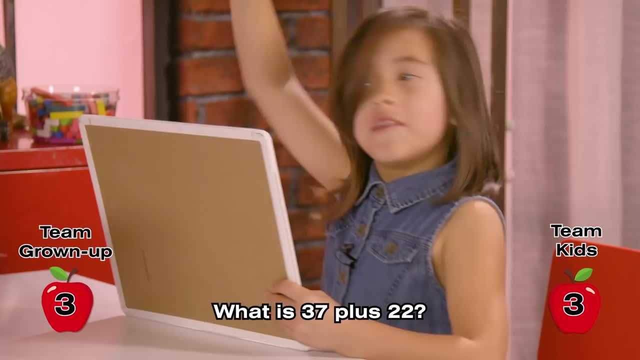 It might be a 2 there. Wait, 6 minus, And this is what grade: 59. 59.. Woo, You're quick, You're quick on your toes. Me, on the other hand, Practice Um, um, um, um 7.. 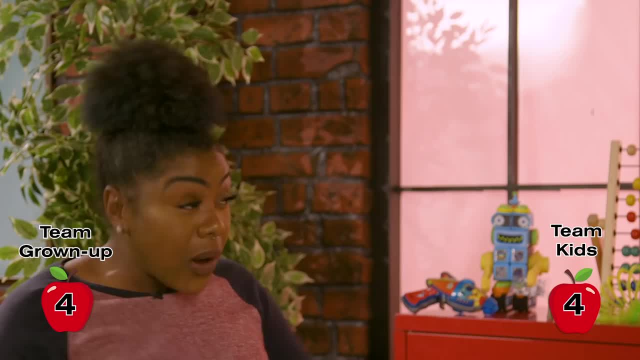 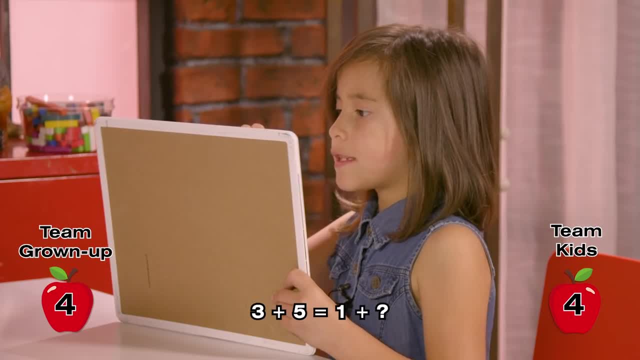 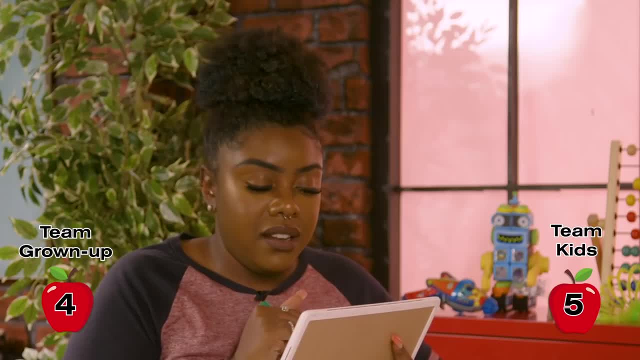 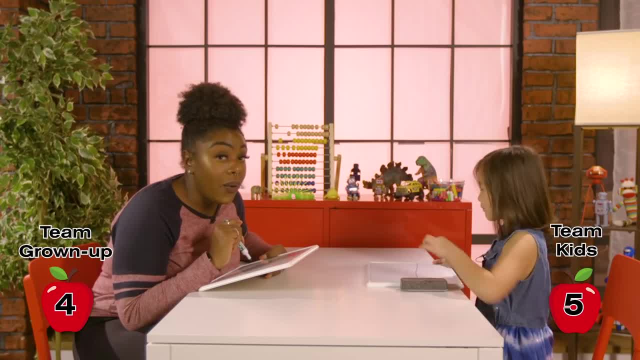 1, 2, 3.. 1, 2, 3.. 1, 2, 3.. I got it One plus 7.. Correct, Oh, really Yeah, Oh wait, No what. 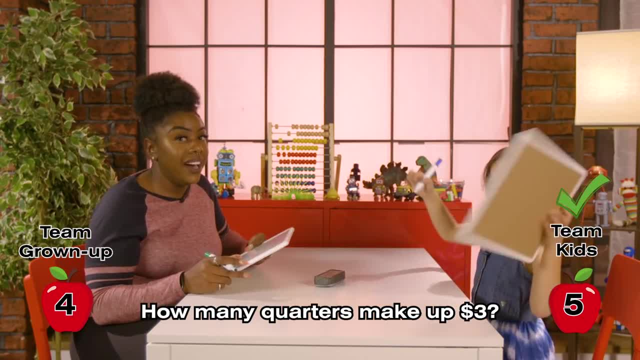 So 3 plus 5 equals 8,. so one plus 7 equals 8.. Oh, That's where I started wrong. How many quarters make up three dollars? Okay, Twelve, Twelve, twelve, twelve, Wow, wow, wow. 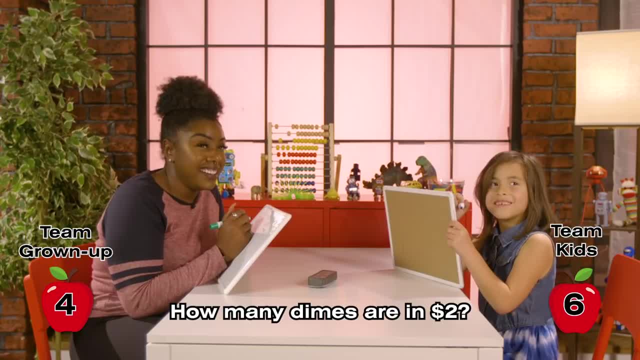 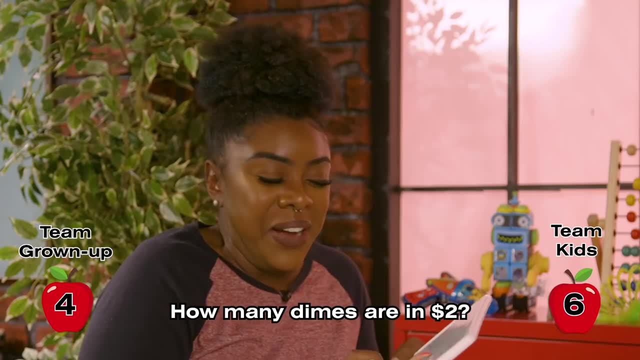 I got to. 4 quarters equals a dollar. All righty, Third grader, All righty. How many dimes are in two dollars? Oh, I got it. Is it 200?? 20!? It's 20!, You did 200!. 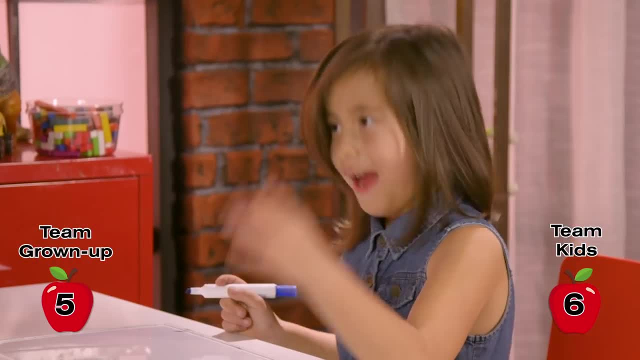 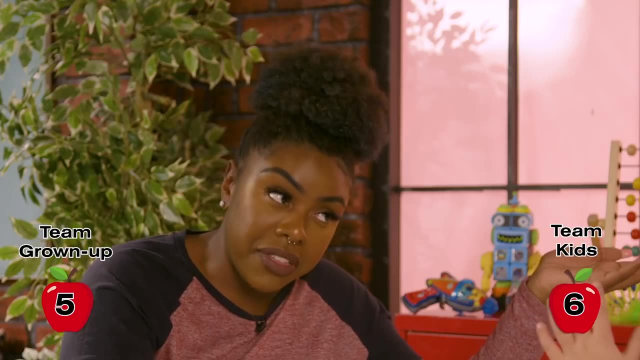 I know. but then I came back: Oh man, That's pennies. I know, I know, I know. That's why I came back and said 20.. I feel like that should count for something, right? Okay, so 12, and then two. 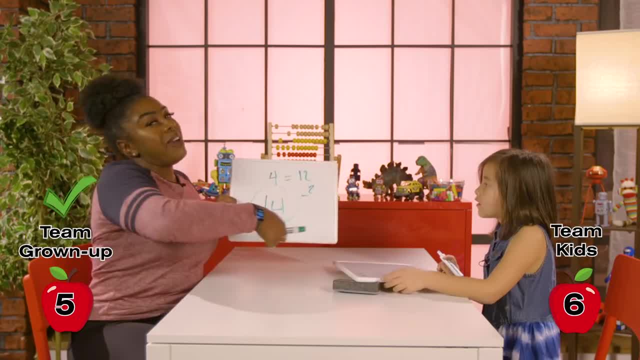 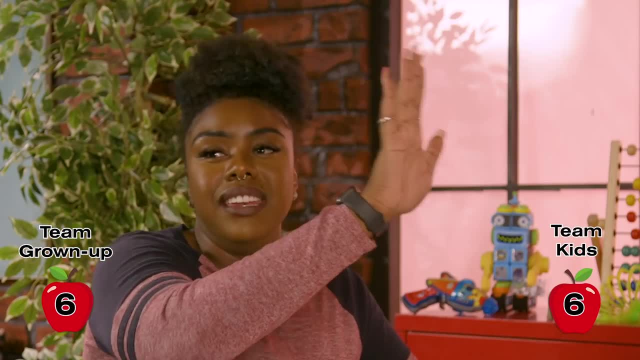 So um 14!. She did the math out loud. it helped, We did it. it's high. What is it y'all are leaving me hanging? What? why are y'all so intense? What is in this cafeteria food? 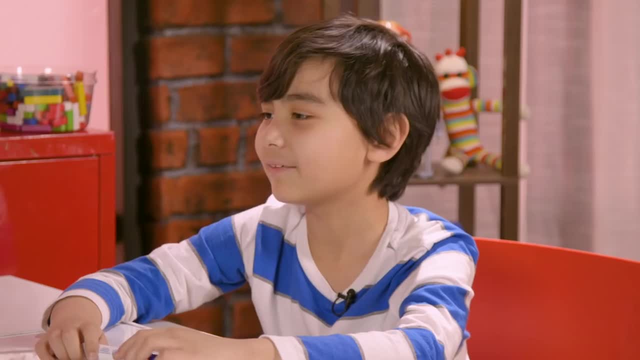 Hi, I'm Destiny. Hi, I'm TJ. Hi, TJ, what grade are you in? Fourth, Fourth, woo, All right, work's cut out for me. then This is like: oh, you're gonna do it, You're smarter than a fourth grader. 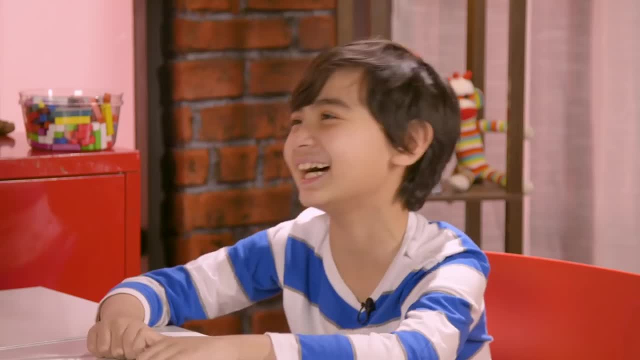 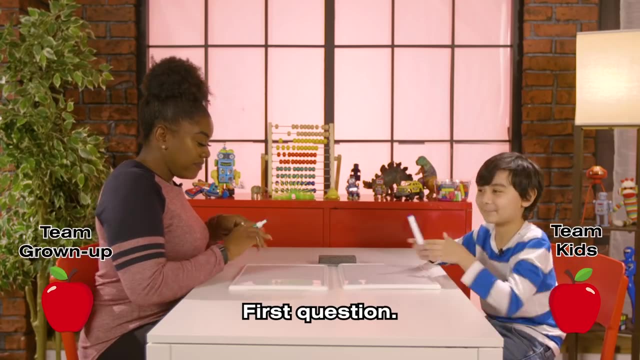 Yeah, and I'm. I don't want the internet to know if I am. All right, let's go, let's get into it. Are you good at math? Yeah, Yeah, okay, Why not? First question: No cheating. 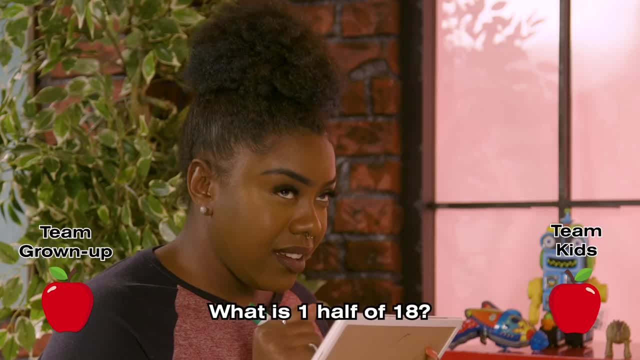 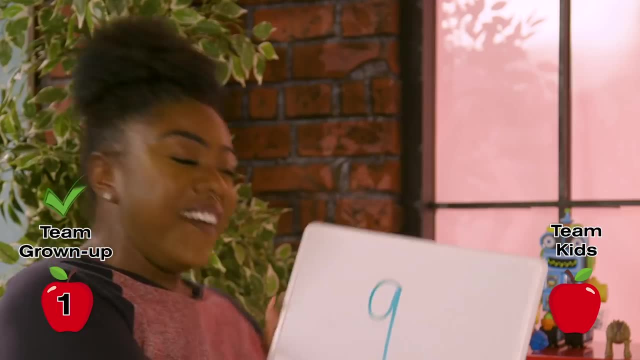 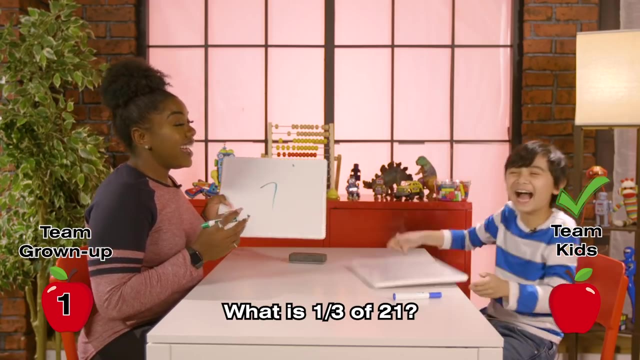 I'll give you one half of 18.. Okay, ooh, Destiny. Ooh, is it nine? It's nine? Okay, One third of 21.. Seven, Oh, I had a lot of preparing to do. What did you say? what did you say? 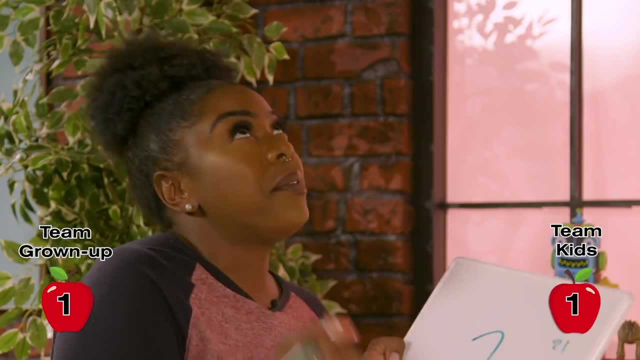 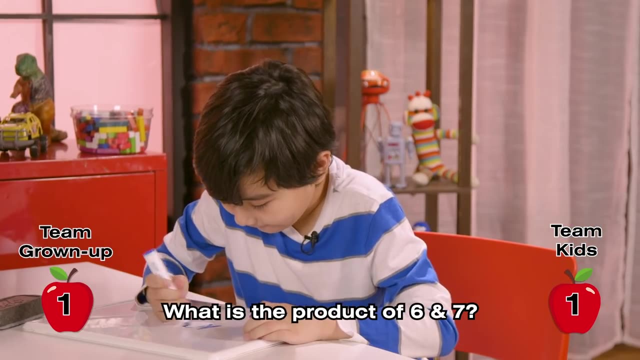 I said seven, but I was like one, third. okay, I need a third of 21.. Okay, one and three times. I'm like: okay, What is the product of six and seven? Answer to everything: 42.. 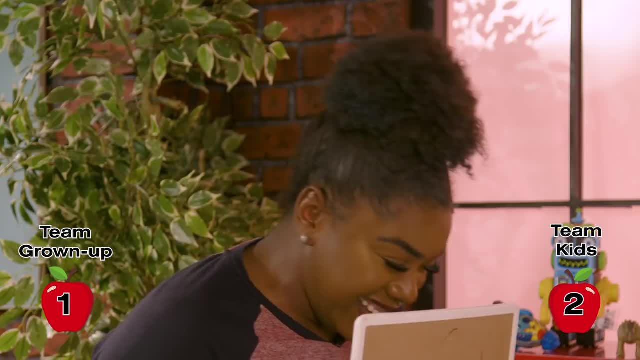 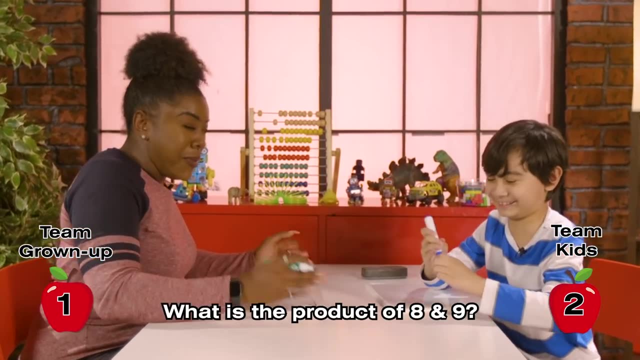 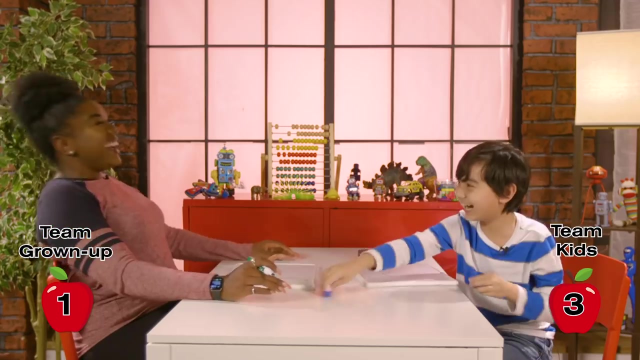 Is that right? Yeah, Oh, my number was off. What was it? I'm not gonna tell you What is the product of eight and nine. Oh, oh, oh, oh, oh, I wrote this so fast. What? 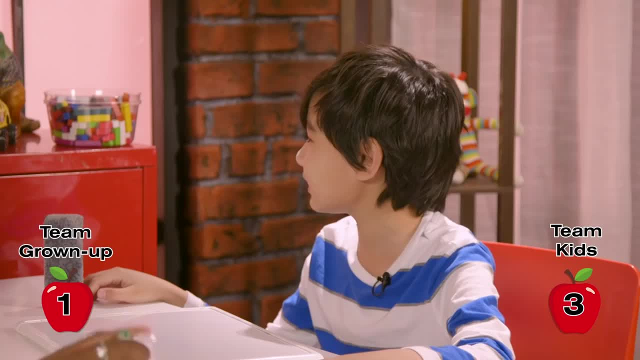 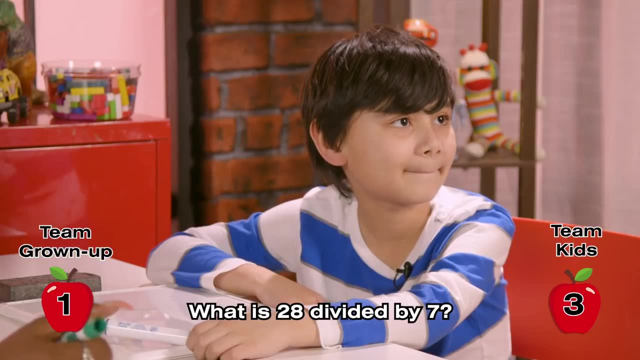 Oh my god, I need time to get there. y'all These toys look like they were invented in, like Europe. Oh you think, Yeah, like what is this block? You just no longer care about the math. What is 28 divided by seven? 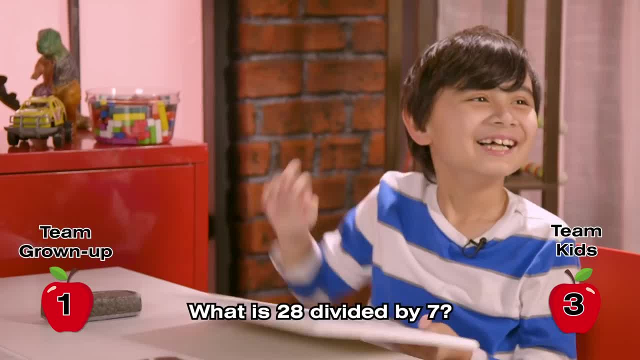 I'm not even gonna answer this, because I put 28 out for something else. Oh see, wouldn't have got it Four. You're so fast with this. Please don't take back my degrees, y'all. I promise, I promise. 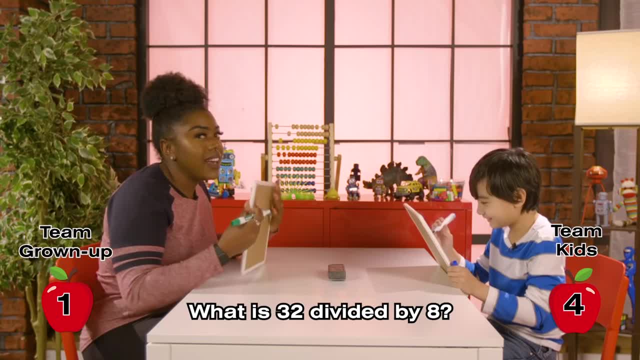 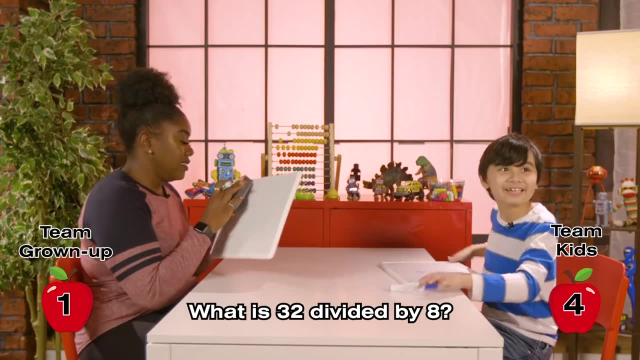 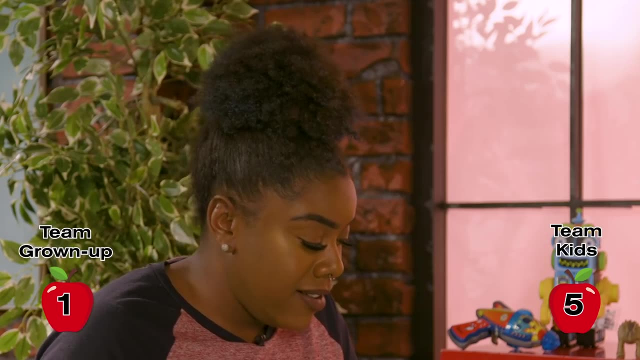 What is 32 divided by eight? I don't know. I'm just gonna put something because I didn't do it last time. Is it six? Okay, I just said something. four: What I don't like this game. I don't like this game at all. 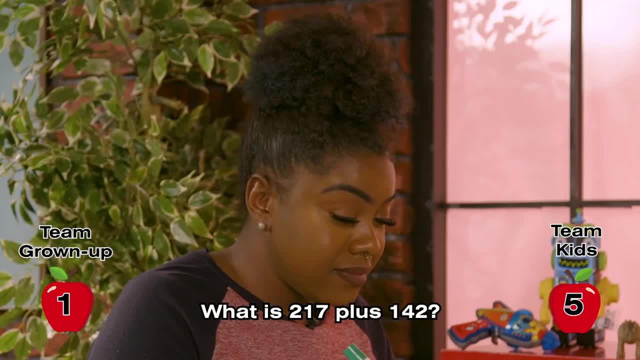 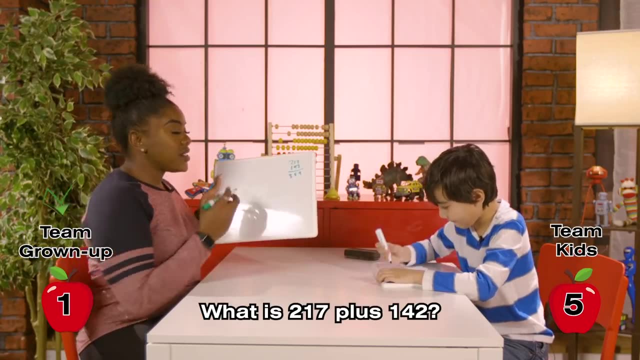 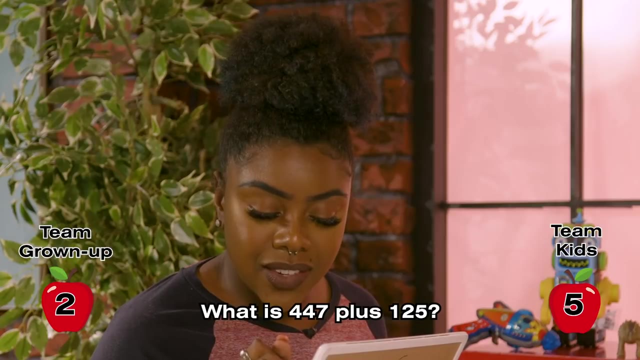 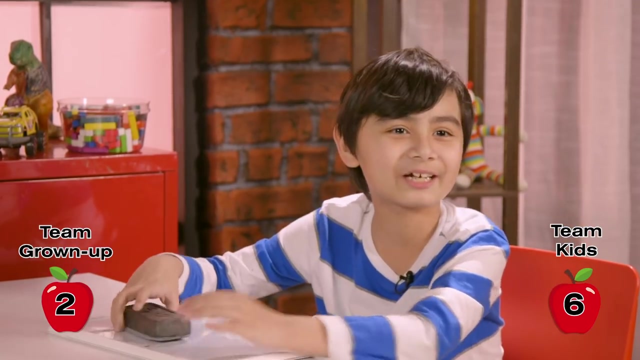 217 plus 142.. That's it 359.. Also sorry it's so tiny, I could do addition. I need to add up bills 572?. You know what I wrote? I wrote six instead of seven and I forgot to regroup the one. 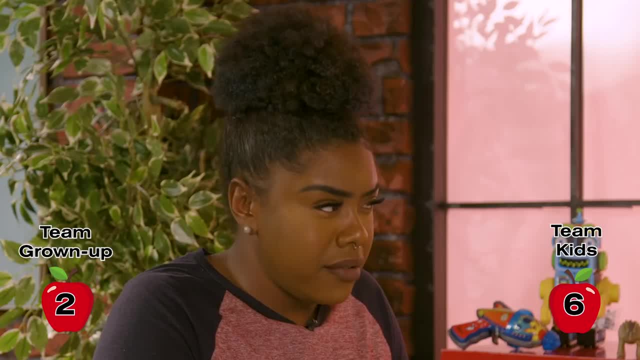 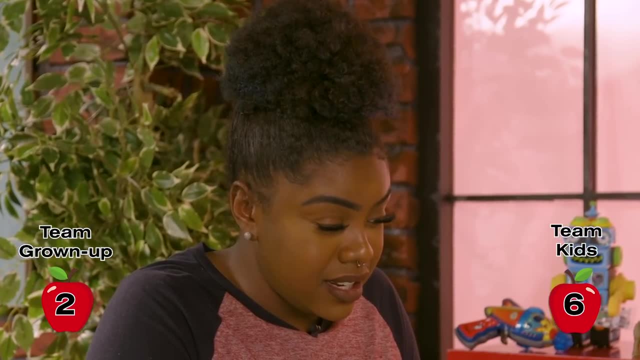 Regroup. You know what regrouping is? No Well, regrouping is when you have, say, for example, seven plus five, You need to put the last digit and then put the next one on the next one and then put the one. that's regrouping.